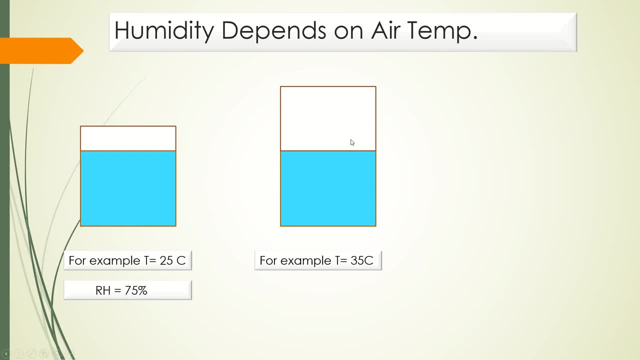 increase. no, the air holding capacity of water vapors increase, so the same water level. the humidity will reduce. so we can say that if the driver temperature or ambient temperature increases, then the humidity will decrease. now, for example, temperature decreases from 25 degree centigrade to 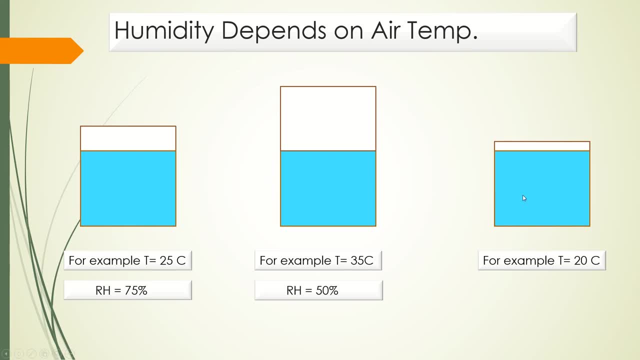 20 degree centigrade, then in this case, with the same water level, the air pocket will decrease. that means cooler air has lower capacity to absorb the water vapors. so in this case humidity will increase. so let's repeat again: by increasing temperature humidity decreases by decreasing temperature. 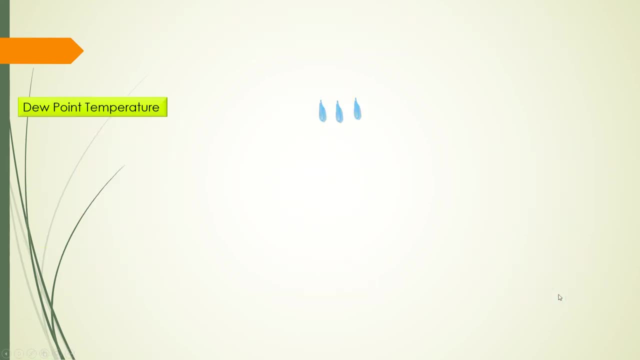 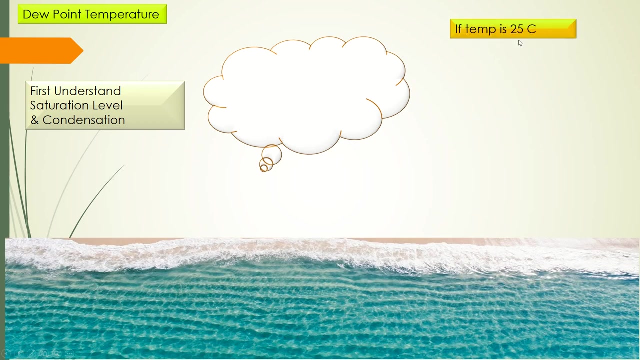 humidity increases now. so before understanding dew point temperature, first we need to understand what is saturation level and condensation. for example, this is again an air holding pocket and this is water. so when? and temperature? you can say that 25 degree centigrade. so when evaporation occurs, then the saturation level of air increase and, as you can see, 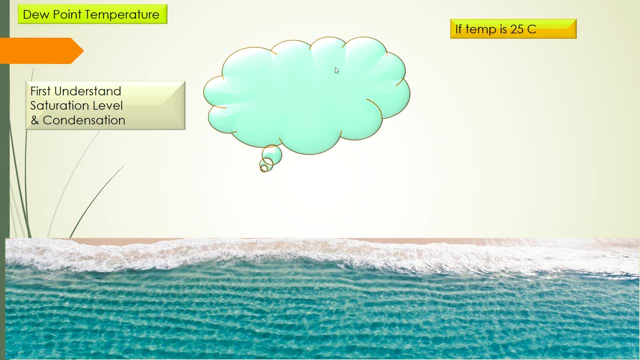 that the whole air is now mixed with with the water vapors. that means air has no more capacity to absorb the water vapors. that means saturation level achieved means no water vapors could be added more. if i affect water vapors, then what will happen? condensation will start. so, guys, i think saturation level and condensation is now. 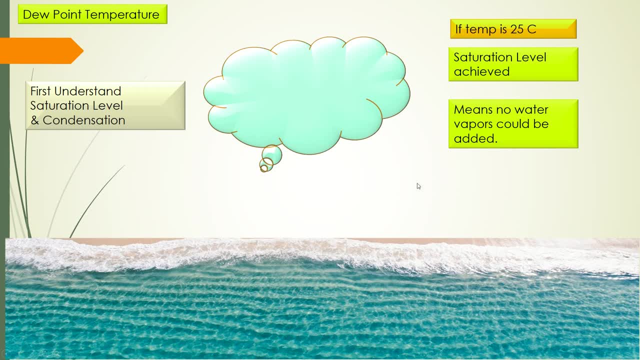 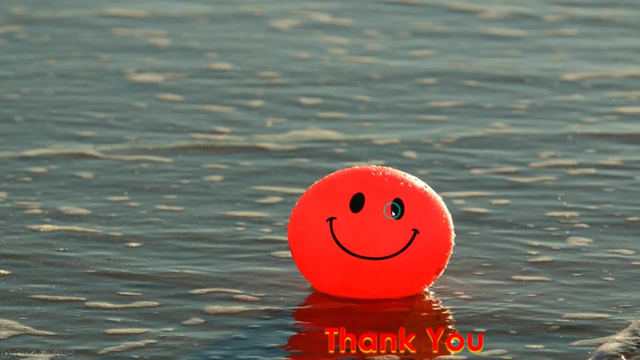 easily understandable now. what is dew point temperature? when saturation level of air achieved, then the temperature of air is the dew point temperature. i hope, guys, you like this video. if you like this video, please share this video and subscribe to my channel. share in your comments. thank you so much.